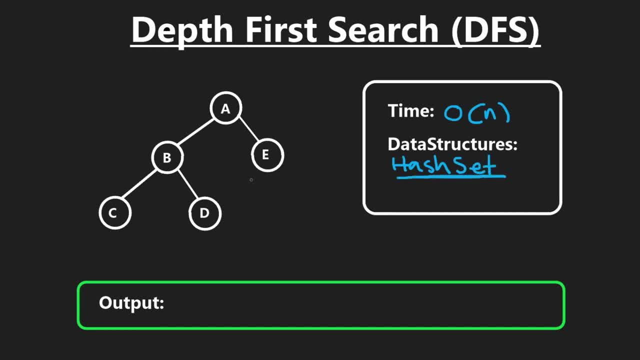 sum. So the hash set is specifically to basically detect a cycle, because depth first search is about traversing a graph. So, for example, if we start at this position, we want to traverse the graph, We go to the next node, we go to another node over here. Suppose these two nodes were 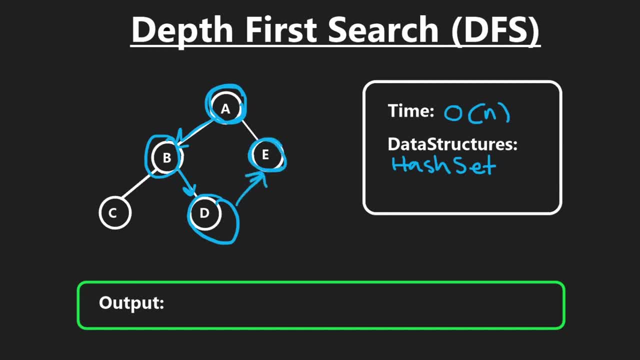 connected, then we'd travel to this node, and then we'd get here and then we'd travel back to this node, which would get us stuck into a cycle. right Now, we don't want to stay stuck in this cycle forever, which is why hash sets are required in many cases. 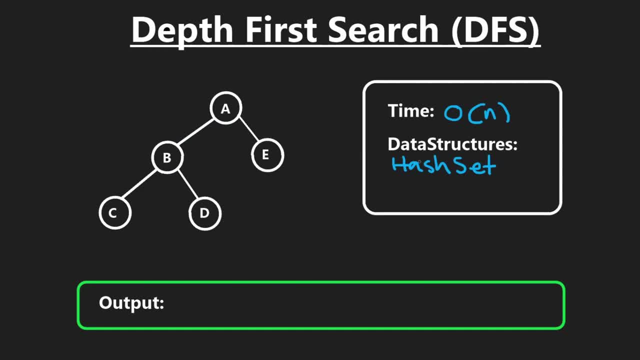 For the DFS algorithm on a generic graph. If you are doing this recursively, you will not need a stack because the recursion handles that for you. But if you do not do this recursively, you can optionally decide to use a stack for DFS problems. Now let's suppose we were doing a DFS on this graph. let's 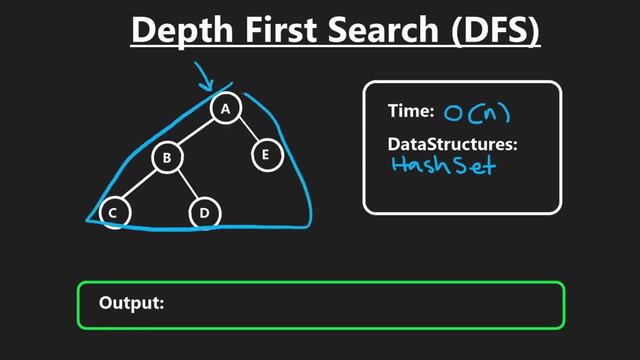 say, starting from A. Now, obviously this looks exactly like a tree and yes, it is a tree, but we know that trees are just special cases of graphs, So this is still a generic graph. Now, if we were starting here at this A node and we were doing a DFS, what would be the output? 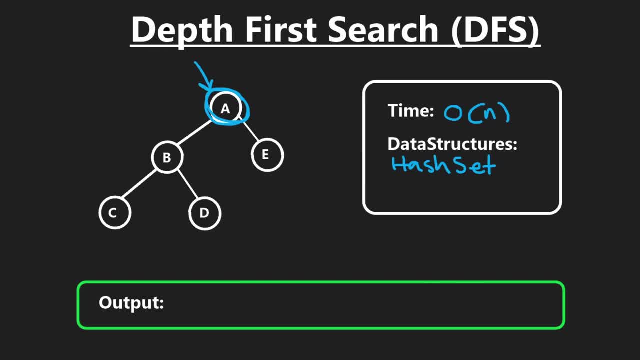 Well, the output, we'd first process the first node, we'd get an A, then we go to the next node. right Now DFS works basically going depth first. So it's depth first. So we do B now, Next we go to C. You can see that this is definitely depth first. We're going as deep. 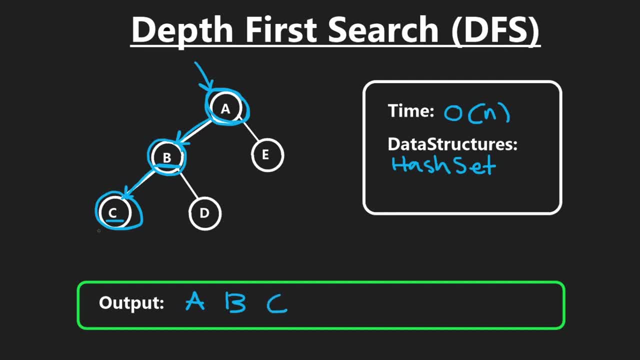 as we can in one direction. So we get to C now. Now we can't go any farther from C, left or right. go back up and we go to the next node that was available to us, the farthest down depth, first right d, and now there's no more nodes anywhere left over here, so then we go to the next node. 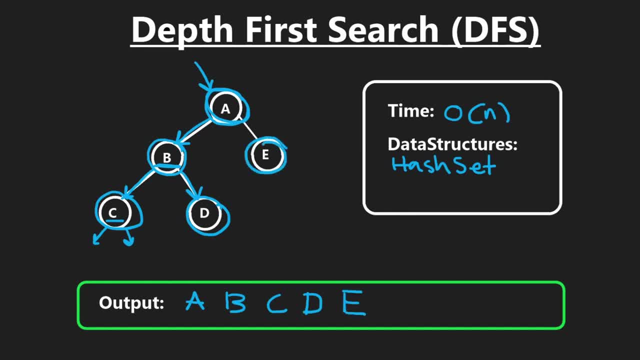 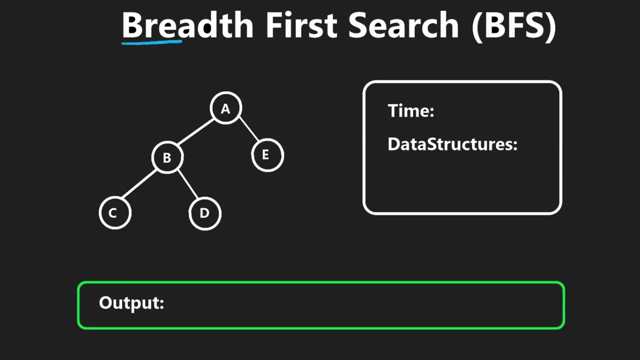 that was available, which was e. we have done the entire graph and this is the output: abcde. next, let's go to our second algorithm, bfs, or breadth. first, search, and, as the name implies, this is also a searching algorithm, which is basically designed to traverse a graph. now this is going to be. 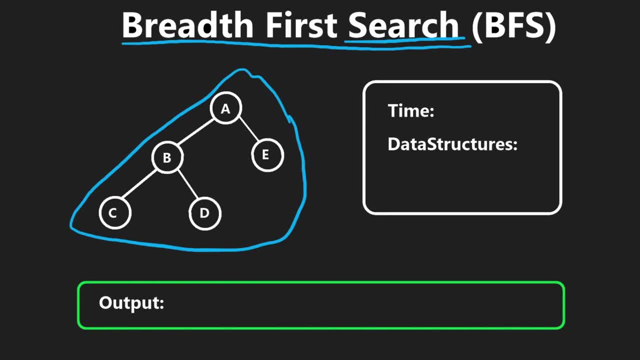 slightly different than depth. first search mainly in the order that it traverses the values, which is what we're going to see when i show you the output: how d bfs would traverse this graph. but the time complexity actually of this graph is going to be the same as dfs, because we're going 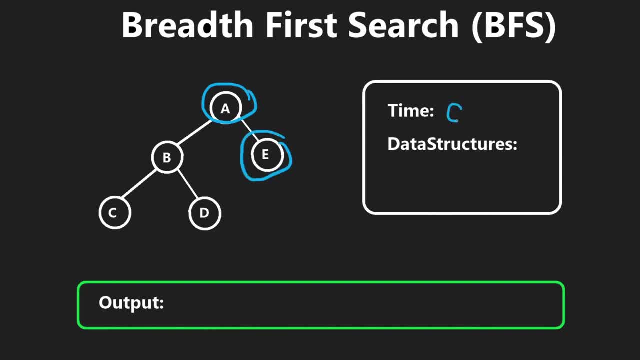 to visit each node at most once, so the time complexity is going to be big. o of n, where n is the number of nodes in dfs, the graph, the data structures typically needed for this algorithm, and it's usually not implemented recursively, so it usually requires a q data structure, a double-ended q, usually again in. 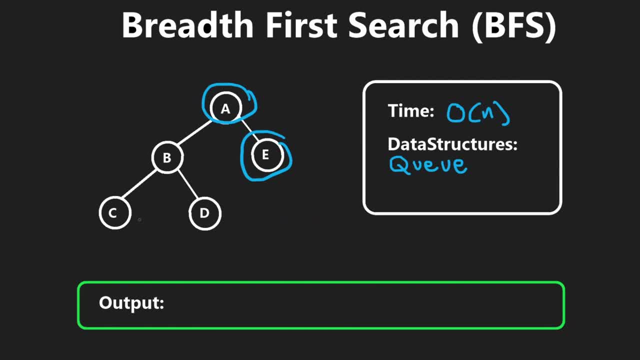 in our graph we could have a cycle similar to the dfs case. so we don't want to get stuck in a loop where we go to one node, go to the next node and then just stay stuck in there forever because we don't want to visit the same node twice. how can we avoid that same case, same way that we did in? 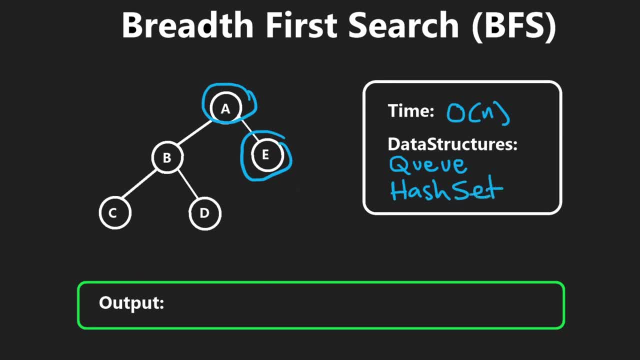 dfs, which is using a hash set to detect duplicate nodes, and bfs is kind of the opposite of dfs. so let's say we start at the same first node. right, we start at a, so let's add a to the output now, instead of going the farthest weekend in one direction. 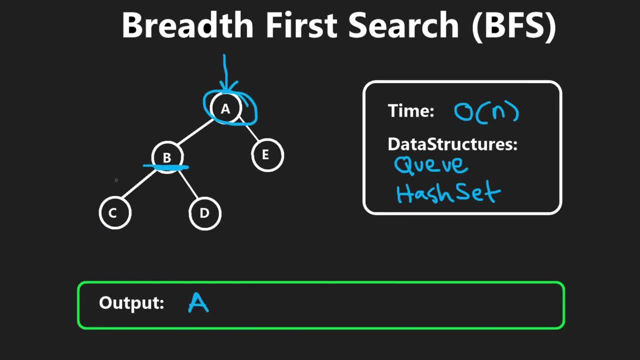 like we did before, like going to b and then going to c. let's do breath first, search right breath, meaning everything that's close to us. basically, we're going to do this layer first, right, we're gonna. we're gonna traverse this entire layer and then we're gonna traverse the next layer, going to. 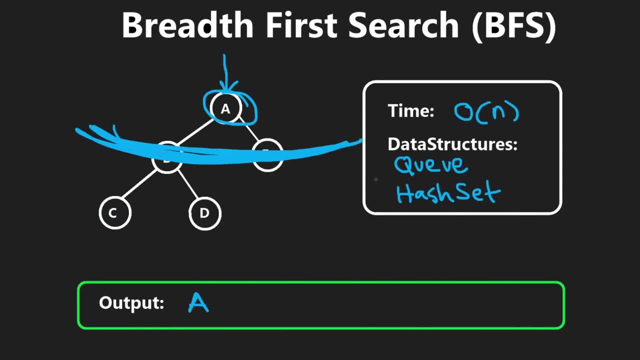 be that truck up in here the graph that's gonna be doing all the work. now that, alright, let's look at the the graph surname and we'll get some information about this graph when it's the kind of working in a next layer and then keep doing that until we run out of layers to traverse. so let's go, let's first. 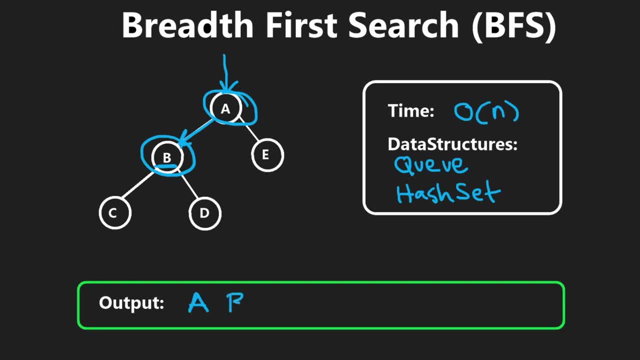 go to b, so b is going to be processed, adding it to the output. then let's go to e, adding this to the output, and you can see that this is a different output than we had when we ran dfs. so this is a different ordering that we're going to traverse these nodes in. so we've done the second layer. 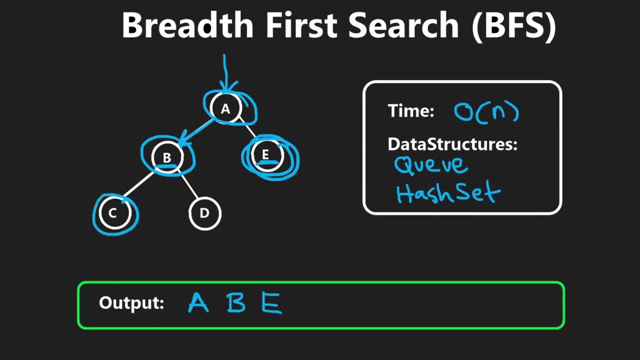 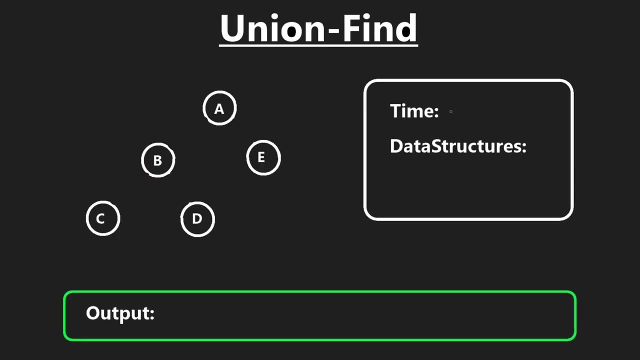 over here. let's do the next layer over here. so we'll do c and then d. so let's add c and d to the output and then you can see everything has been processed in the entire graph. we had a slightly different output than we did with the dfs case, so the third graph algorithm is definitely a little. 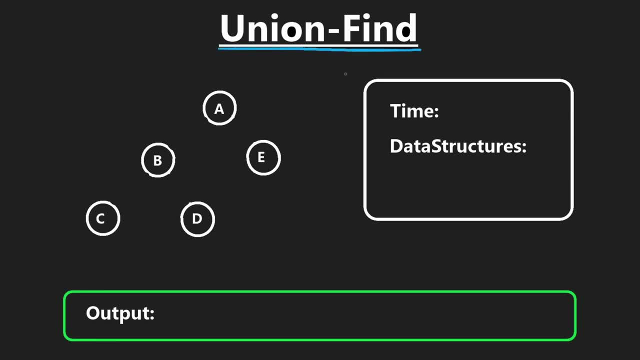 bit different. this is union find, which is used to kind of union together, disjoint sets, and kind of combine them together efficiently. so the overall time complexity of this algorithm is usually bounded by n, log, n, and in terms of data structures, what i'll say is that we've got a lot of data here that we need to go through and we need to go through. 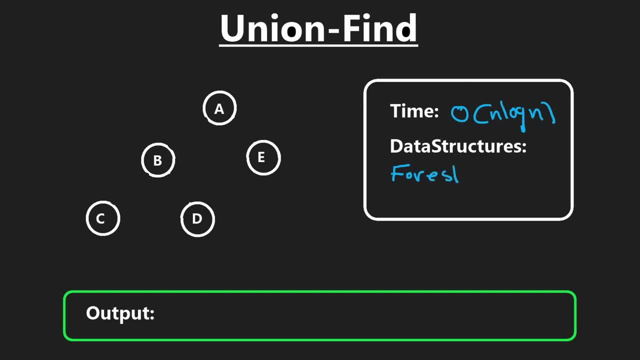 a lot of data for that to be clear. so i'm going to go through this and then i'm going to do this and is just that it requires basically a forest of trees, which is really how I was taught how this is implemented. But basically you usually have to implement union. find yourself. The good thing is. 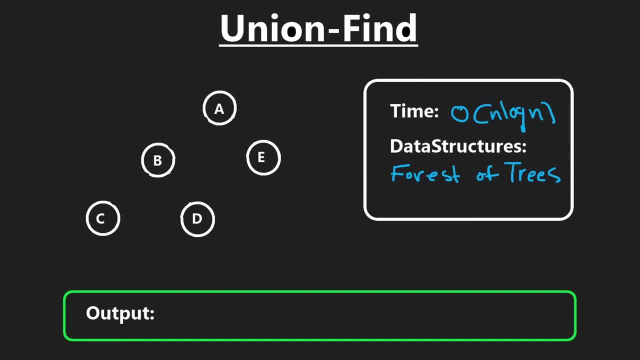 it's not super hard to implement it Because, for example, one thing we could do with union find is basically what if we wanted to know the number of connected components of a graph and we were given five different nodes? Now, of course, in this case, we have five connected components each of these. 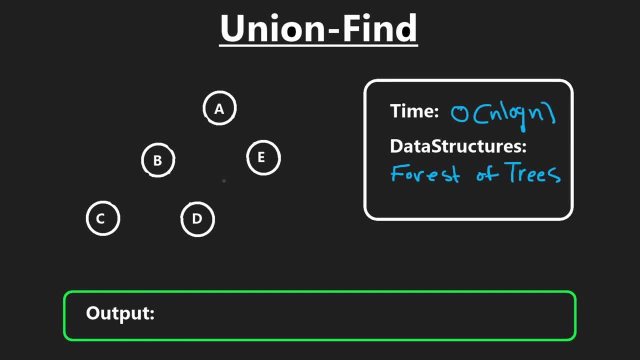 is a component now. But what if we start arbitrarily adding edges? If I say, okay, I'm going to add an edge here, I'm adding one edge, Well, that decreased the number of components from five down to four. Now, now we only have four. What if I take another edge and increase it? 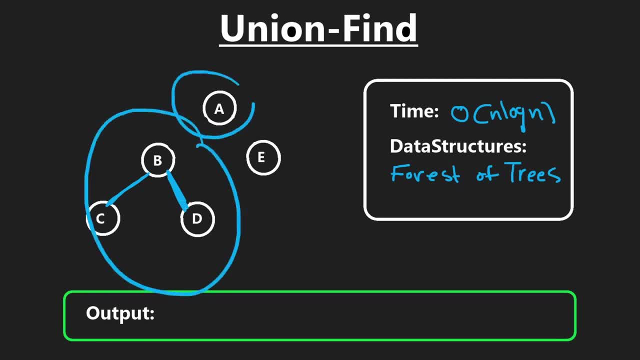 or add the edge over here. Now we have three different connected components. What if I take another edge and add it over here? Well, that didn't change anything. we still have one, two, three, three connected components. Union find is basically an algorithm that can do stuff like 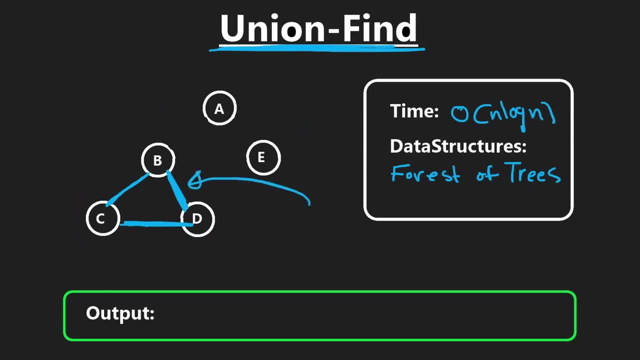 this efficiently for us. So suppose we added these three edges. Now we want to know how many connected components we have. We have three connected components, exactly three. So three would be in the output. Now this is a very high level overview. If you would like a more detailed, 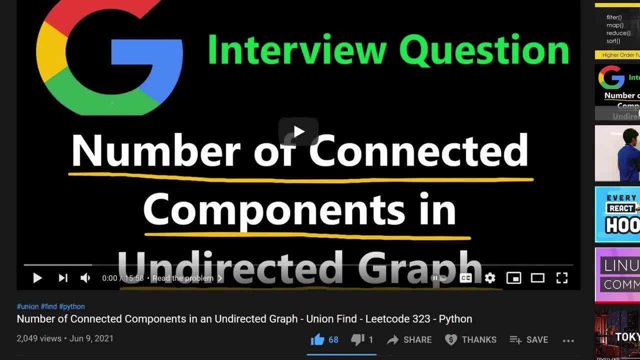 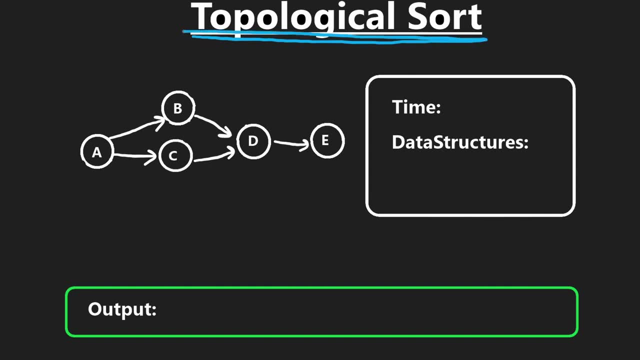 explanation of the union find algorithm. I would recommend watching this video, which is actually number of connected components in an undirected graph which we solved using union find. So the next algorithm on our list is definitely one of the more difficult ones and definitely more obscure. You don't see this algorithm used a lot, but it is topological. 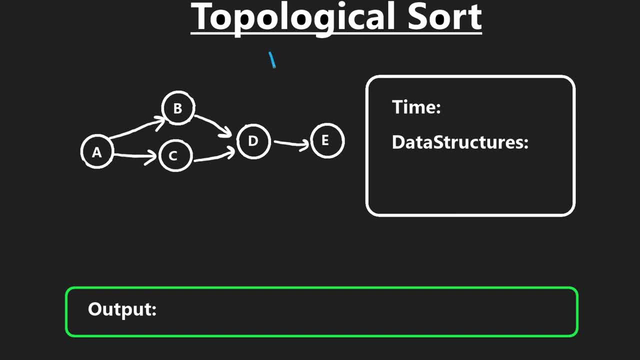 sort, And this algorithm is actually built on top of one of the previous algorithms, DFS. You can see why DFS is so important: because it's actually used in a lot of other algorithms, including topological sort. So topological sort, basically, is a algorithm that can do stuff like this. It can do stuff like this. It can do stuff. 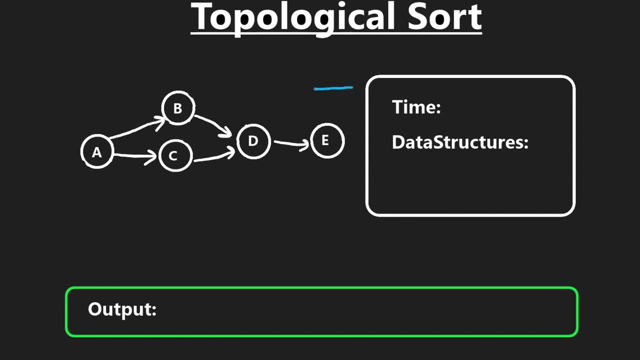 at a high level is we are given a directed acyclical graph, basically a graph with directed edges, and the graph will not have any cycles. Basically, the topological sort of a graph like this one would be reading the values of every single node in the graph, but only basically. 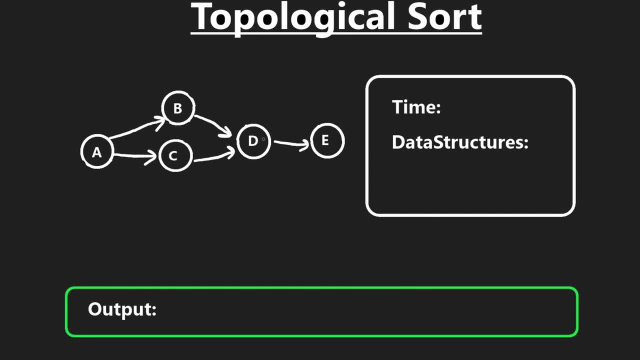 printing those values out in such an order that, for example, D when we print D, we have to make sure that every node that came before D, we have to make sure that every node that came before it has already been printed or processed or traversed or whatever you want to call it. 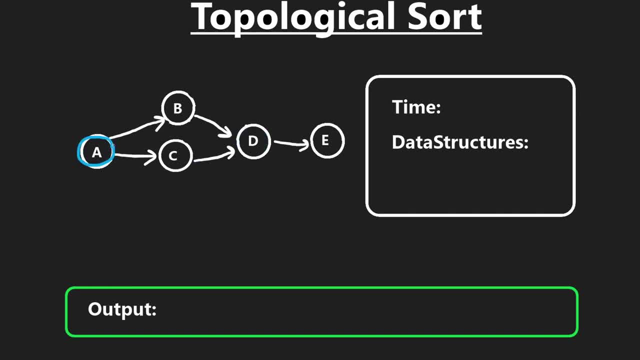 So one valid topological sort would be A, B, C, D and E. A topological sort doesn't have to be unique. There's actually two different topological sorts in this graph. We could do A and then we could do B and then C, or we could do C and then do B. That's two different choices we have, But 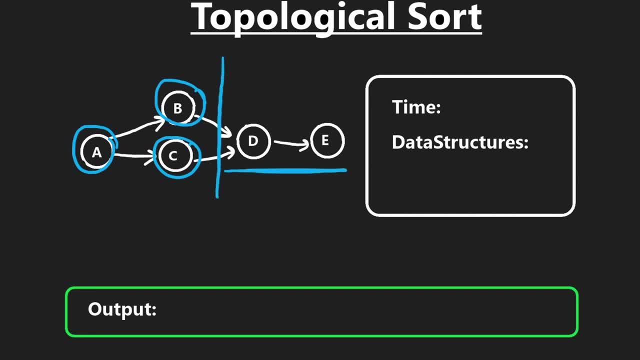 once we do those, then the choices are limited. Then we have two nodes left. We have to do D before we do E, So one topological sort could be A, B, C, D, E. We are doing this with depth-first search, so the overall time complexity is going. 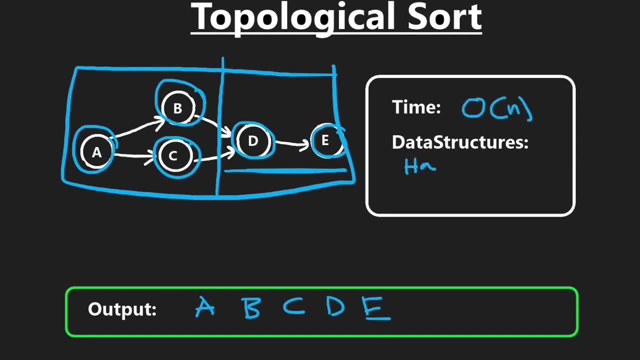 to be O of N. We are going to be using a hash set since we are doing DFS, but if we do it recursively, that should be the only data structure that we actually need. This was a very quick explanation of topological sort, but if you would like a more detailed solution and explanation, 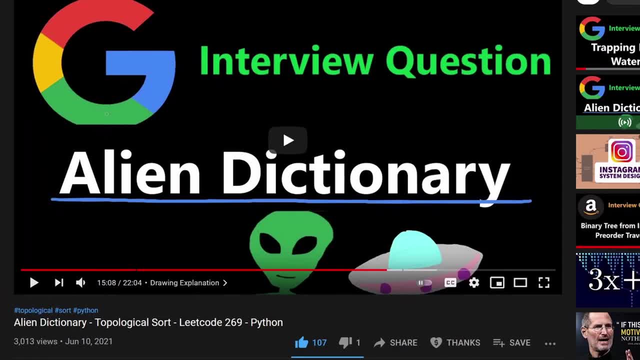 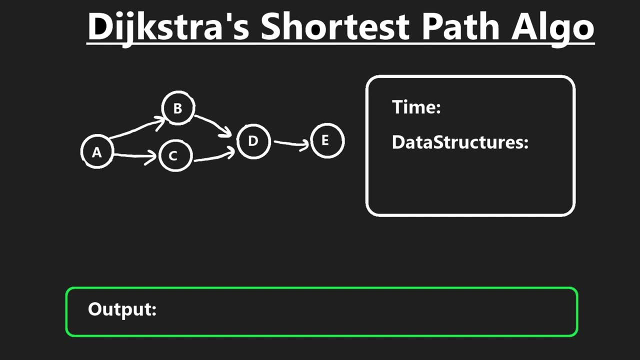 I would recommend you to go to the link in the description below. And the last algorithm I wanted to quickly go over is Jixtra's shortest path algorithm. This is definitely a popular, famous algorithm and it does show up in leetcode, though it's not super. 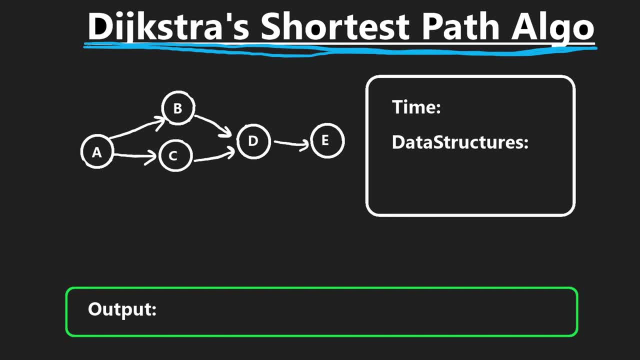 common in leetcode and encoding interviews, but it's definitely a good to know. You'll definitely learn this in school. Just like the name says, it's about finding the shortest path from what you're looking for, So if you're looking for a short path algorithm, then you should. 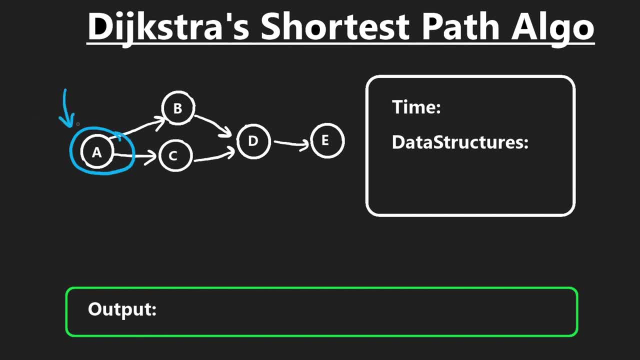 find the shortest path from one node. So let's say we had a starting node A. We want to find the shortest path from A to every single node in the graph A, B, C, D, E. right, We want to find the. 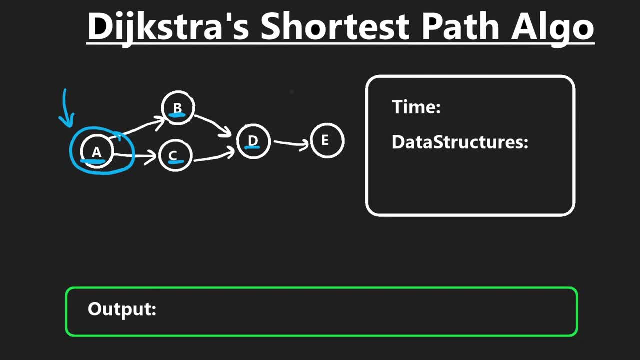 length of the shortest path. Now, the graphs we've been looking at so far have been pretty simple graphs: right. Each edge actually doesn't have any weight associated with it. Each edge basically has a weight of one right, A simple weight, because they're all equal. but we could actually have 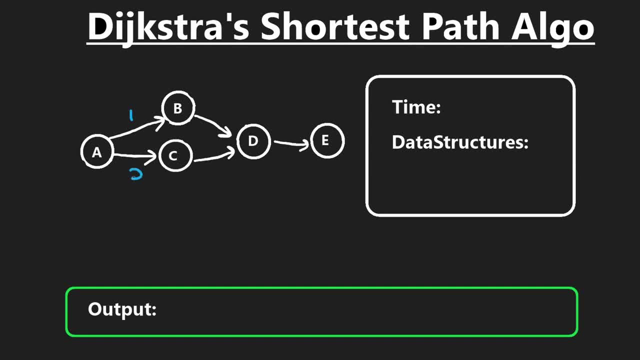 edges of different values. We had something like this, So this makes finding the shortest path a little bit more difficult, because we actually have to look at the values of every single edge in the graph now And the overall time complexity of Jigster's algorithm is actually more complex than a regular DFS. It's. 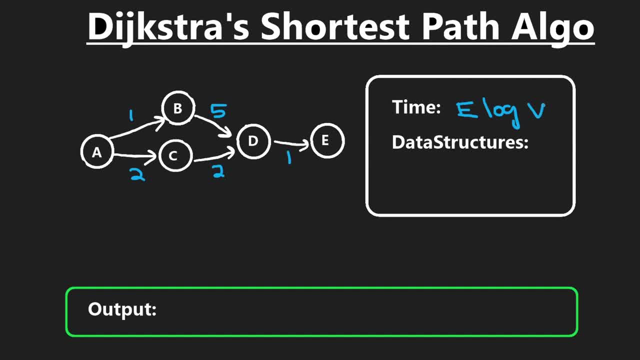 typically E log V, where V is the number of nodes or vertices in the graph, E is the number of edges in the graph. It's a little bit more complex, It's a little bit of a worse time complexity because we have to deal with these edges. Now, how are we going to deal with these edges? What? 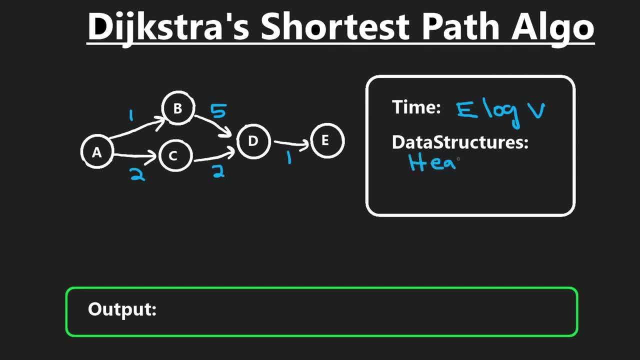 data structure. are we going to use A heap or a priority queue, however you want to call? it is usually the main data structure used to find the shortest path, because we're going to have to be looking at the minimum edge and we're going to have to be looking at the minimum of many 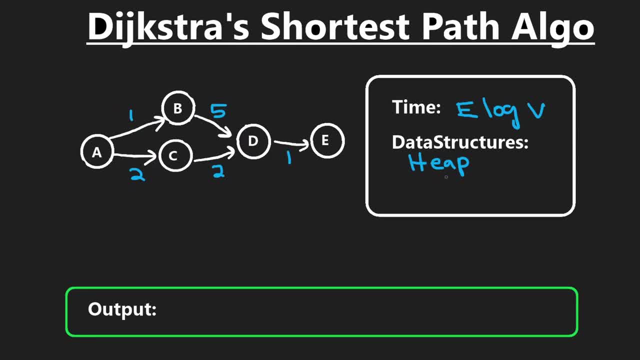 different values. So the heap is going to be very helpful for doing that, And you still don't want to get stuck in a cycle. So hash sets are also helpful for this algorithm. And just to give you a quick rundown of how this algorithm would work on this example: 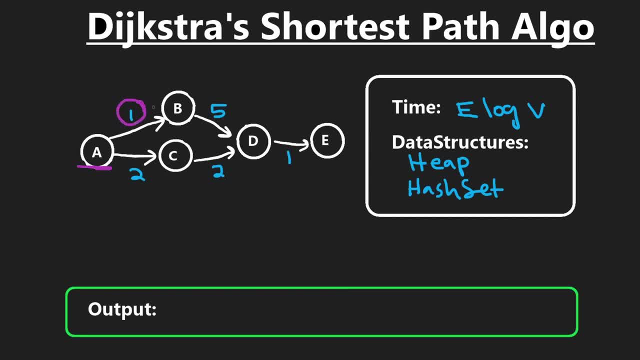 we'd start at A. We'd look at the shortest edge: It's 1.. So then we'd get to B. We'd say you know, the length to get to B is just going to be 1.. Then we'd look at the next two edges that 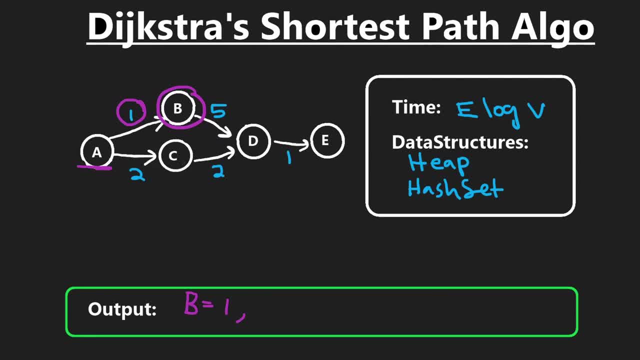 are available to us, We'd choose the smaller one, this one which would get us to C. So we'd say, to get to C, it just takes a length of 2, a weight of 2.. And then we'd look at our next frontier. 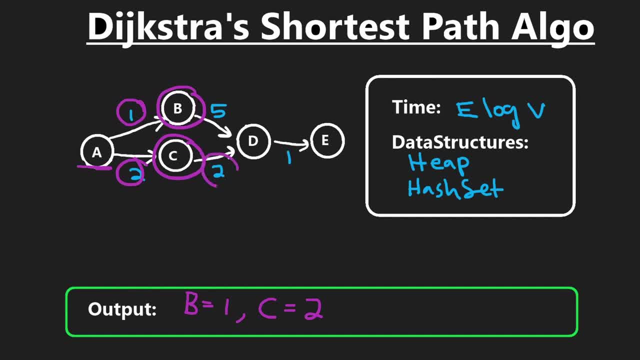 We could choose the 5 or the 2.. Of course we're going to choose the 2.. So then we'd say at this point D: the cost to get to D is actually 4.. We don't just include this single 2, but we also include the. 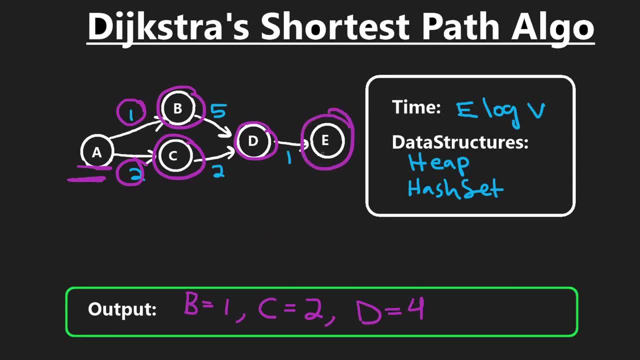 previous 2 that it took, And then the last edge is E, or the last node is E. How long does it take to get to E? Basically, as far as it takes to get to D, which is 4, plus this 1.. So E is 5.. So this: 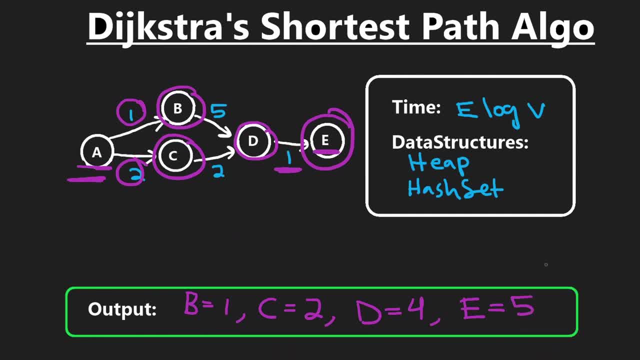 is kind of the you know the shortest paths to every single node in the graph And for a more in-depth look at this, we're going to look at the last node, which is E. So we're going to look at the last node, which is E, And for a more in-depth look at this, we're going to look at the last node.